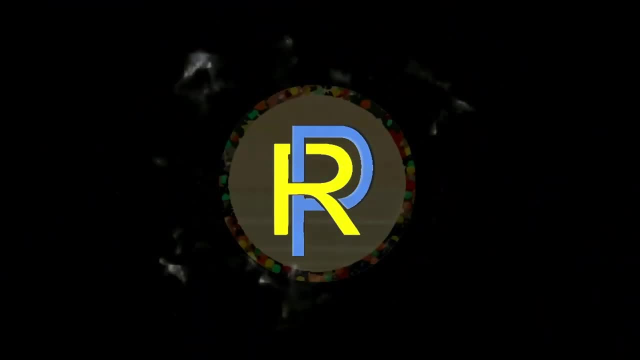 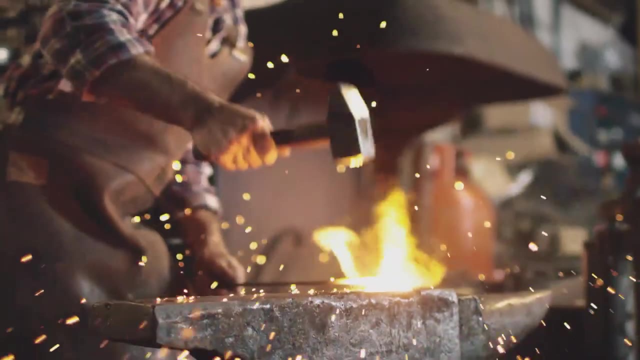 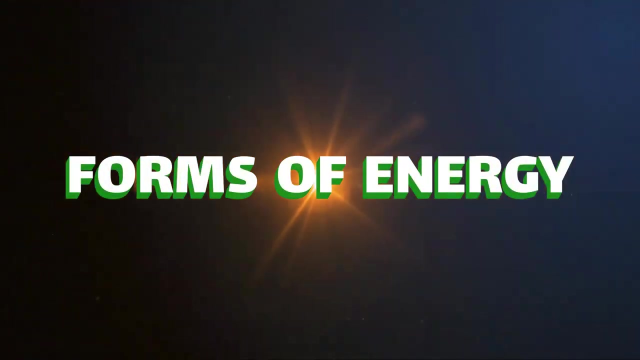 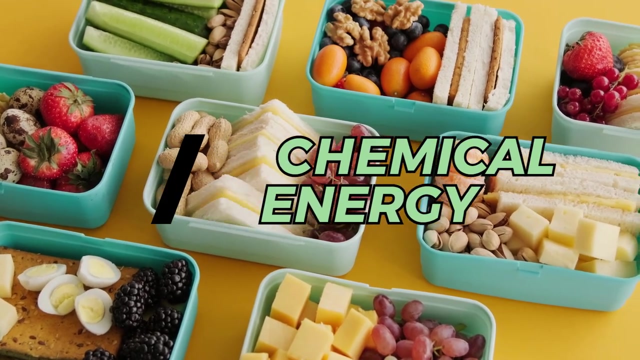 Energy is the ability to do work and produce changes. In this video, we are going to study the different forms of energy. Chemical energy: This energy is stored in some substances such as food or batteries. When you eat pasta, your body receives energy from. 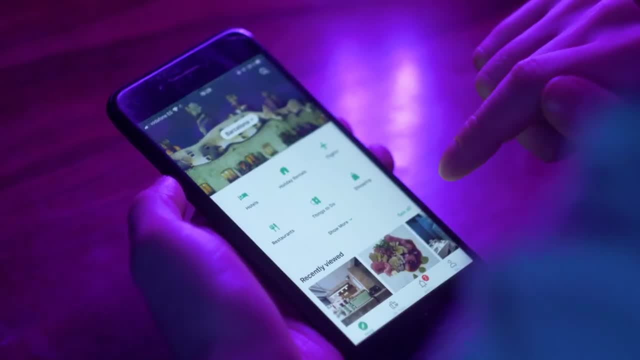 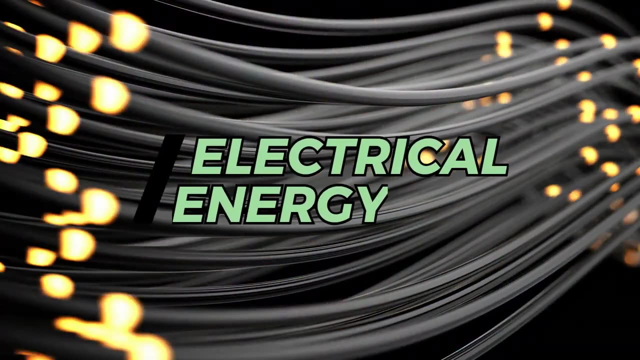 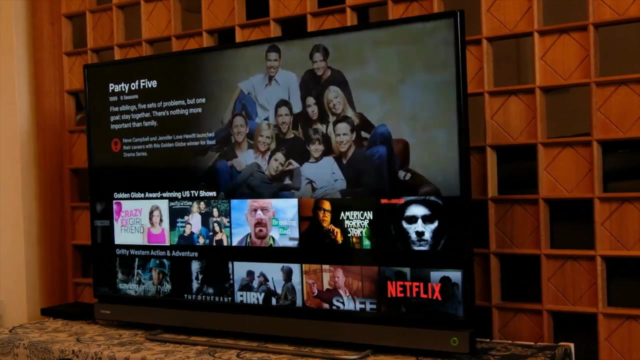 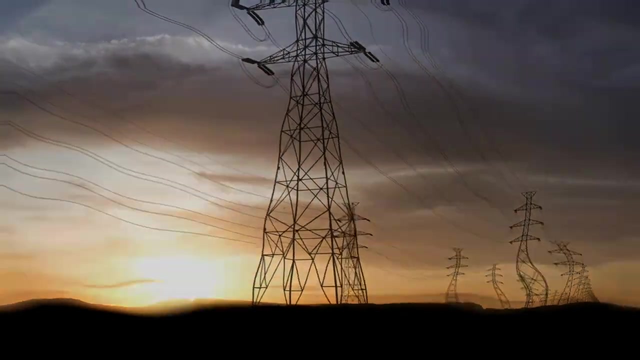 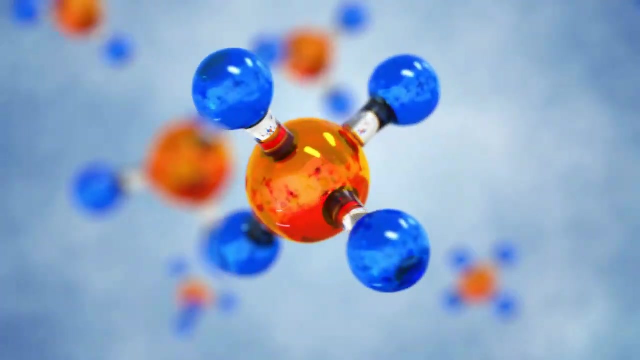 carbohydrates. When you use a mobile phone, the battery transforms chemical energy into electrical energy. Electrical energy: This is the motion of charged particles. For example, televisions use electrical energy. Electricity reaches homes and factories through metal cables. Thermal energy: This energy is related to the movement of atoms in an object or substance. The more movement. 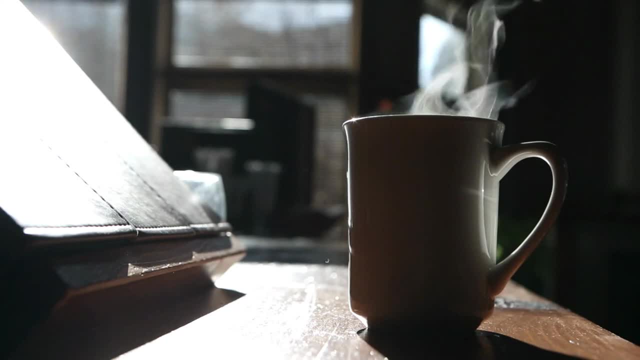 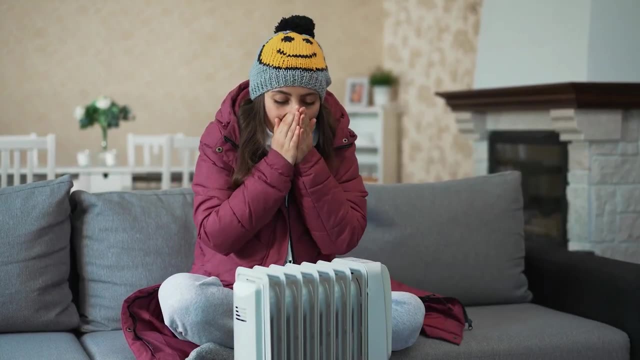 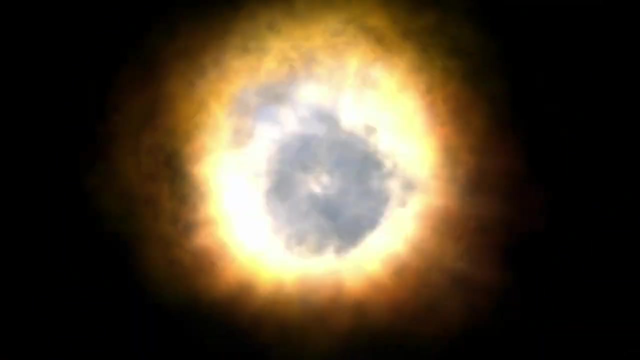 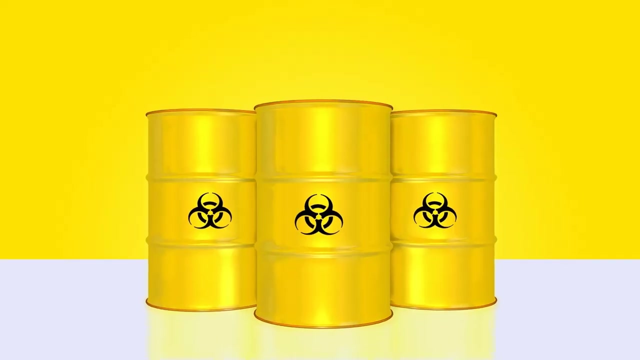 the more temperature and therefore more thermal energy. We use this energy to heat food, buildings and so on. Nuclear energy: This type of energy is stored in the atomic structure of matter. Scientists release this energy by breaking down the atoms of radioactive materials such as uranium. This is done in nuclear power plants. 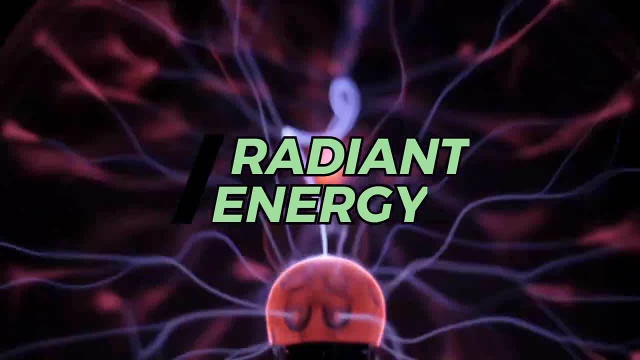 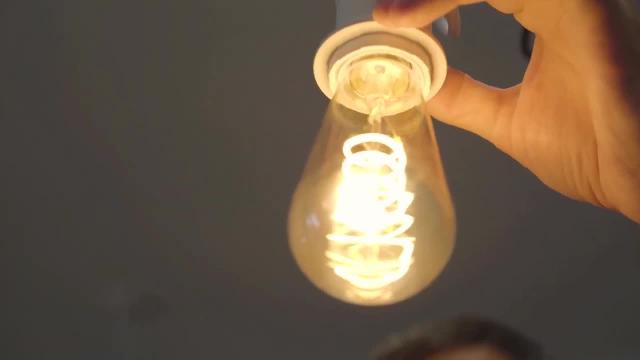 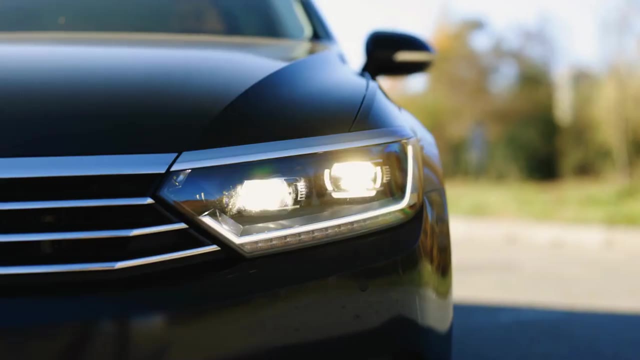 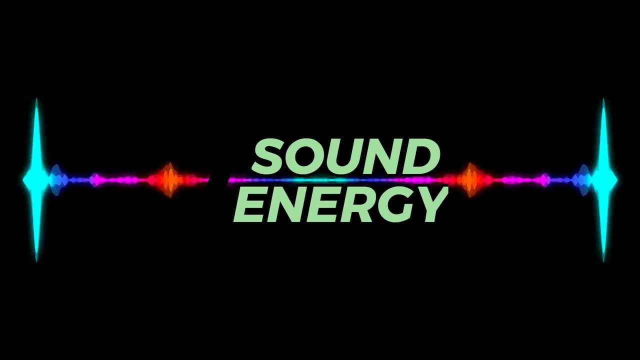 Radiant energy. This is the energy in the form of electromagnetic waves. Light is an example of radiant energy known as light energy. We use light energy in flashlights, cameras, computers, cars or street lights. Sound energy: Sounds are produced by vibrations traveling through air. 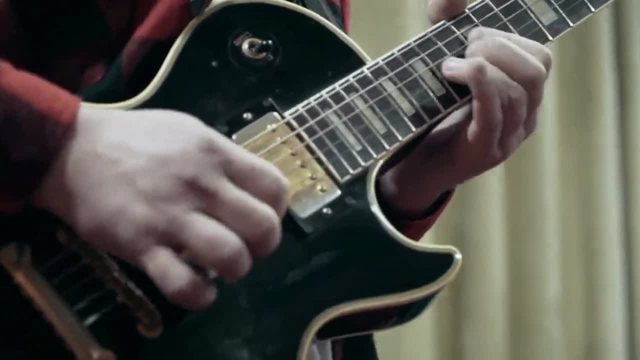 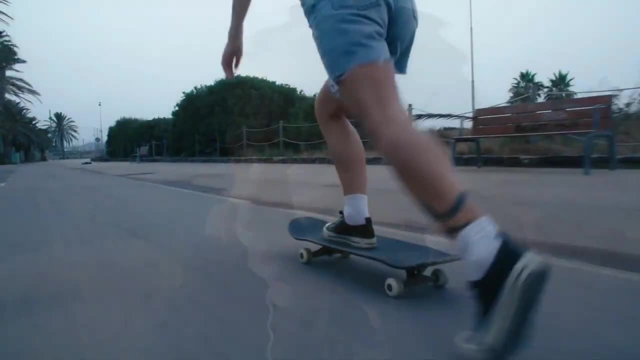 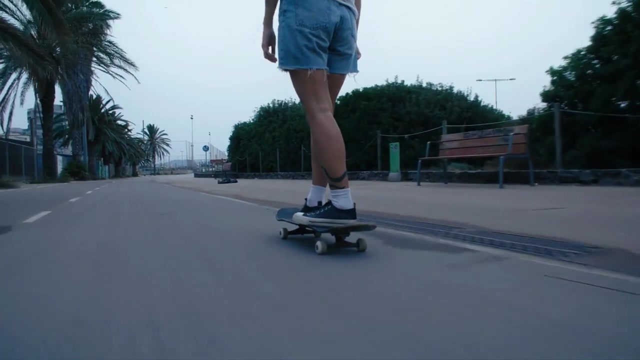 liquid or solid objects. The waves make our eardrums vibrate and this allows us to hear Mechanical energy. The energy produced by motion is mechanical energy. It is the energy that allows people and things to move go faster or change direction.